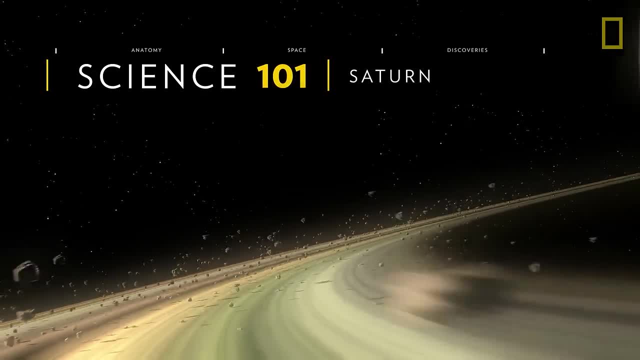 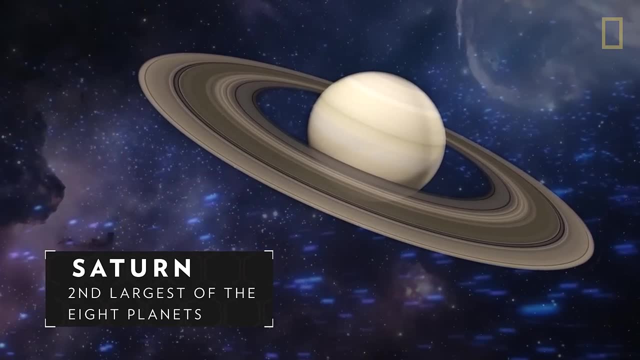 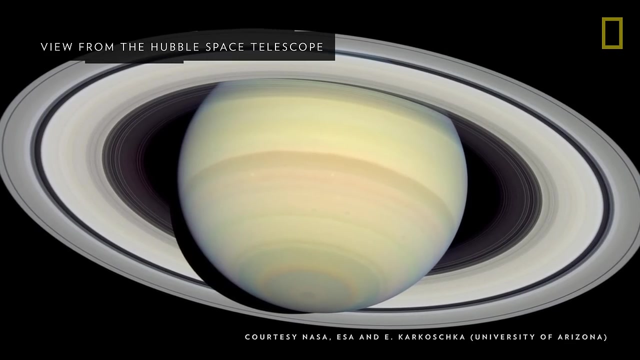 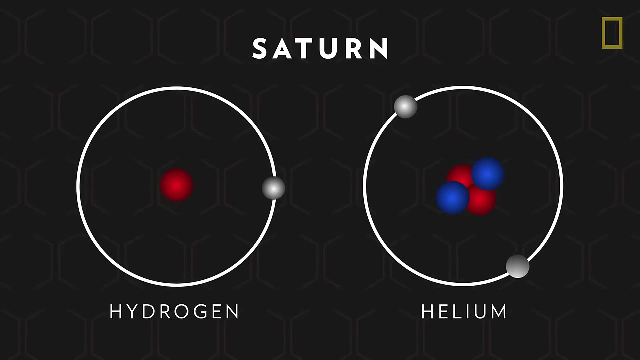 With its gold color and stunning rings, Saturn is quite a planetary gem. Saturn is the second largest of the eight planets and it is about ten times as wide as Earth. Despite its size, Saturn is actually the lightest planet. It is predominantly made of the gases hydrogen and helium and, because of its particular gaseous composition, 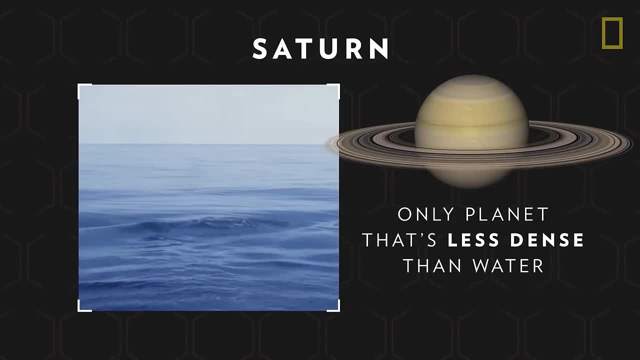 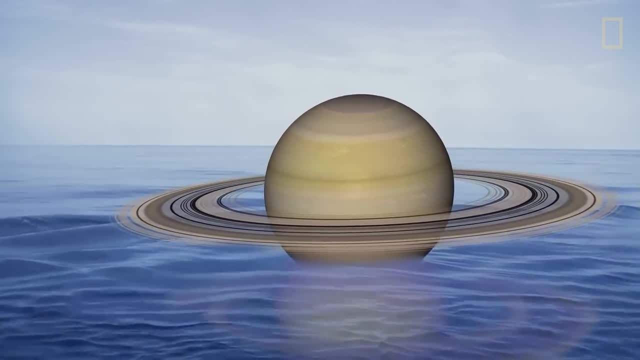 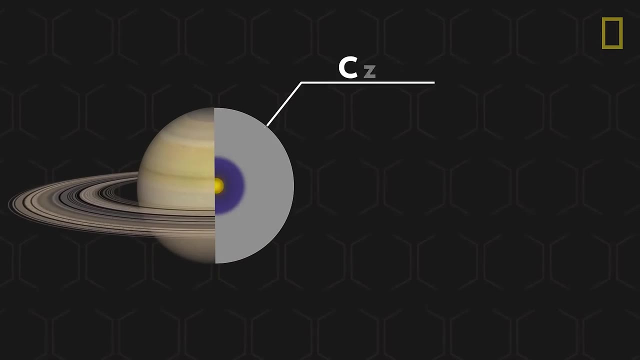 Saturn is the only planet in the solar system that's less dense than water. If the planet were placed on an enormous ocean, it would be able to float. Saturn's gaseous makeup also means that it has no true surface. At its center, the planet has a dense core of water, ice and rocky material, but it has no actual landmass. 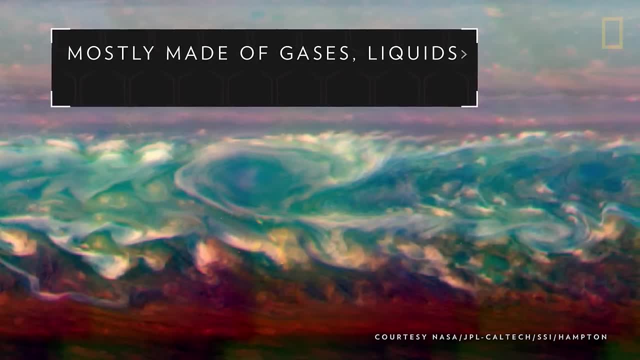 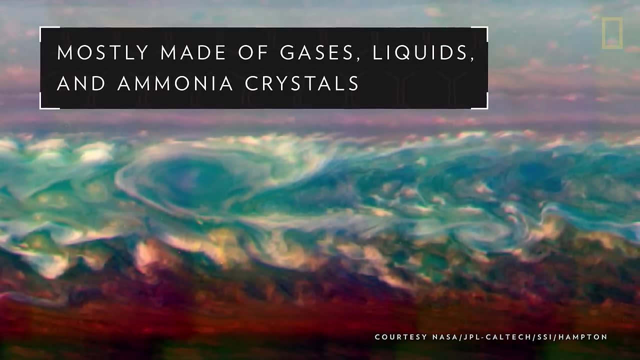 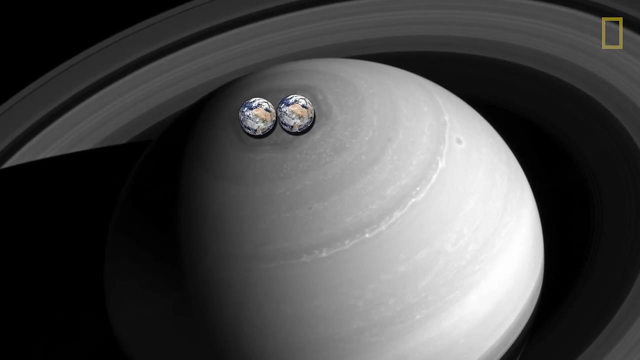 Instead, it's mostly made of gases, liquids and yellow oxygen. These are all ammonia crystals that swirl around the planet, creating golden clouds and storms. The largest storm on Saturn is at its north pole. It's over twice the size of Earth and shaped in a near-perfect hexagon. 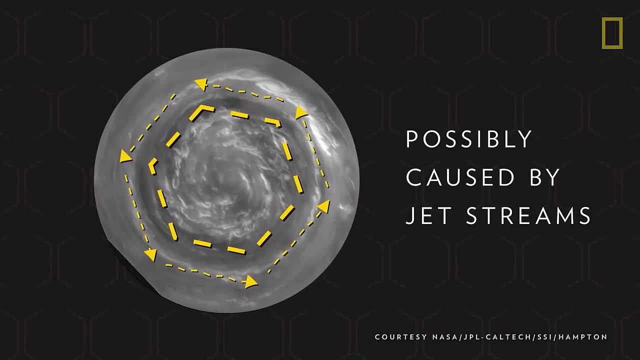 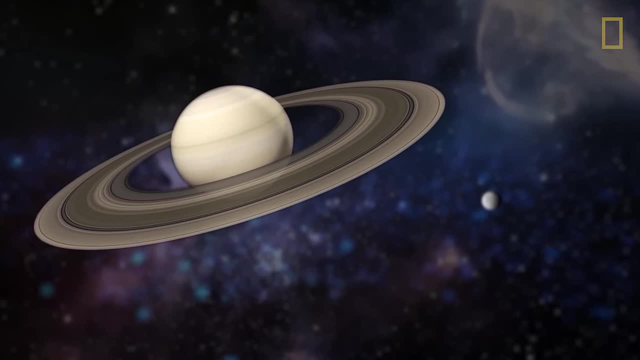 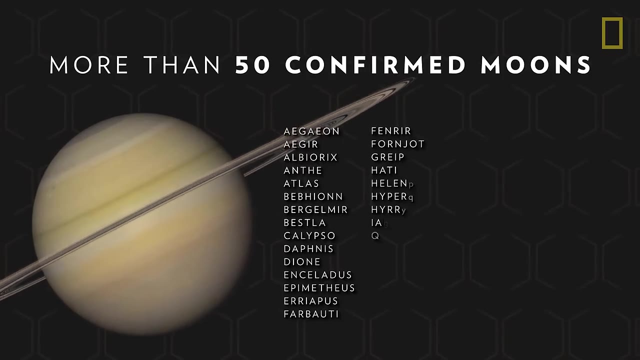 Each of the six sides is believed to be the result of jet streams which all encircle a massive hurricane. Because of Saturn's inhospitable environment, the planet cannot support life, But some of its moons might. Saturn has more than 50 confirmed moons, and each varies in size and terrain. 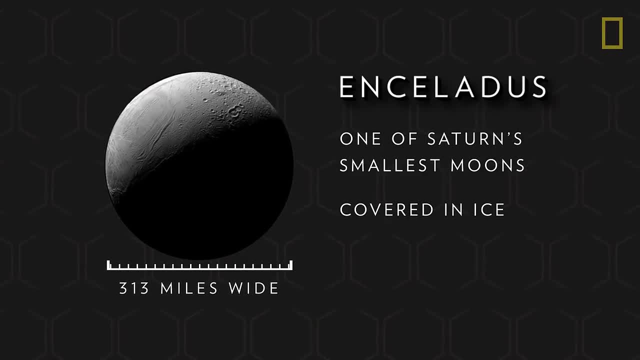 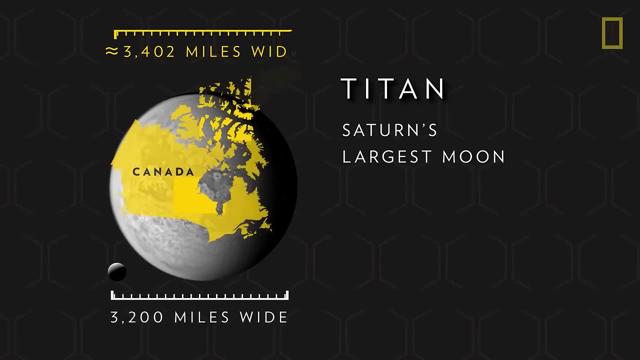 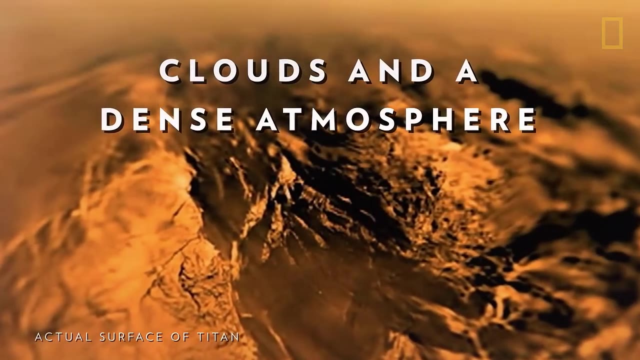 Enceladus, one of Saturn's smallest moons, is covered in ice and only about as wide as the state of Pennsylvania. Titan, Saturn's largest moon, is nearly as wide as Canada. Titan is also the only moon in the solar system with clouds and a dense atmosphere. 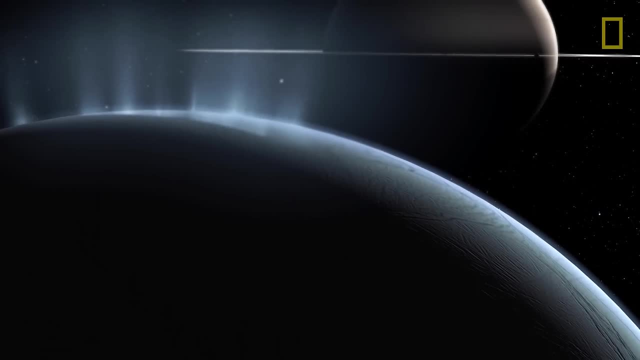 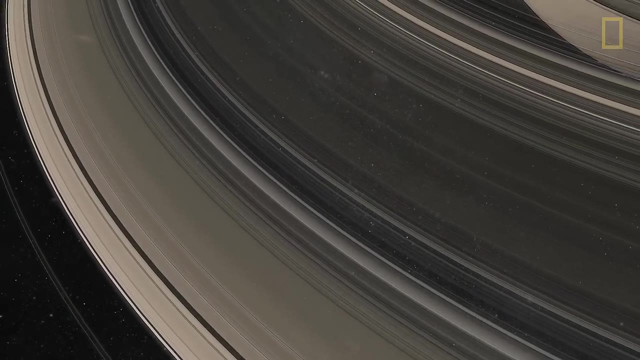 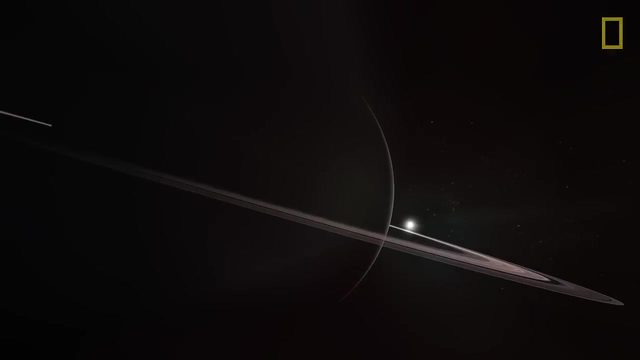 Both Titan and Enceladus have underground oceans that would make them potentially capable of sustaining life. Saturn's moons may also play a role in shaping the planet's signature feature: its rings. Saturn's ring system is the largest and most complex in the entire solar system.